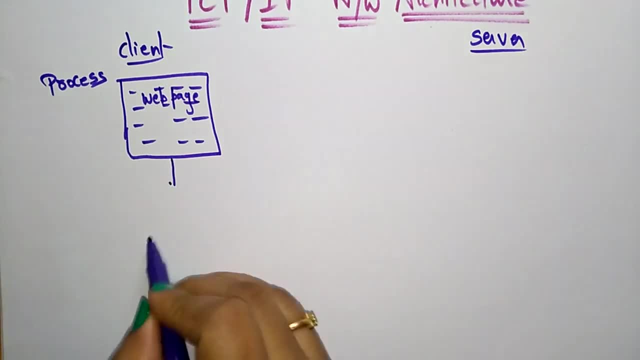 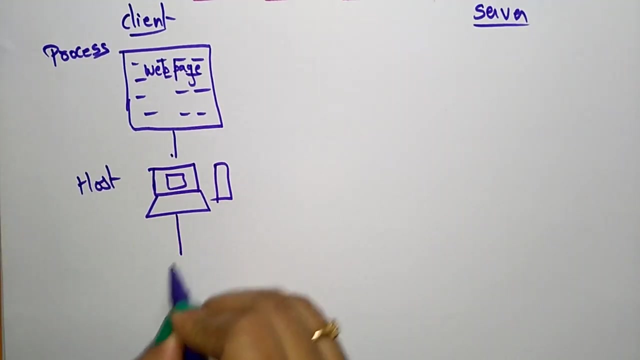 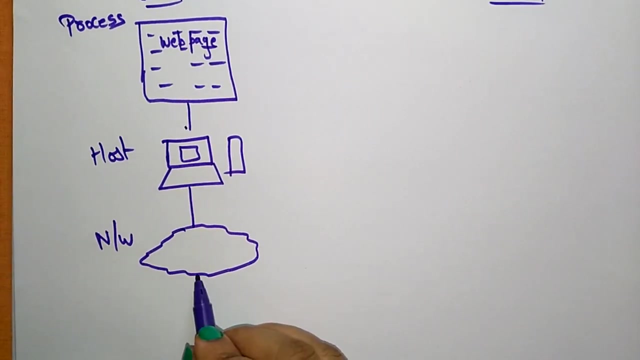 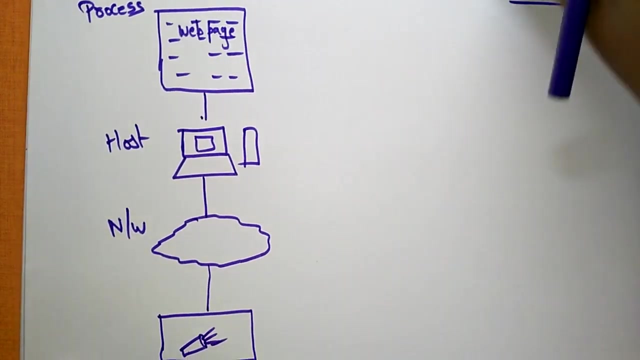 And next this process is going to the transport layer. So, whatever the page I open so that it goes to the transport layer, So the transport layer is nothing but the host of the system. And next it reaches the cloud. That is network. So how it reaches? It reaches the network with the help of cable, So this is a physical cable. So we call it as a media. 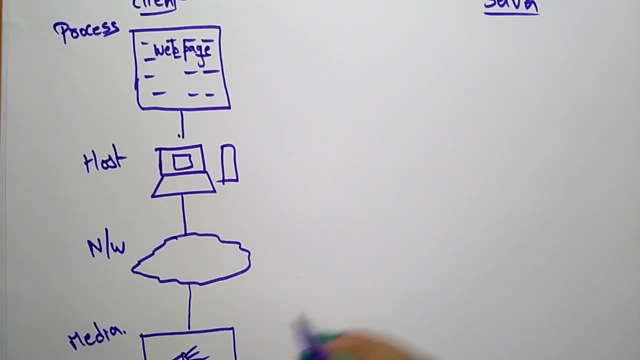 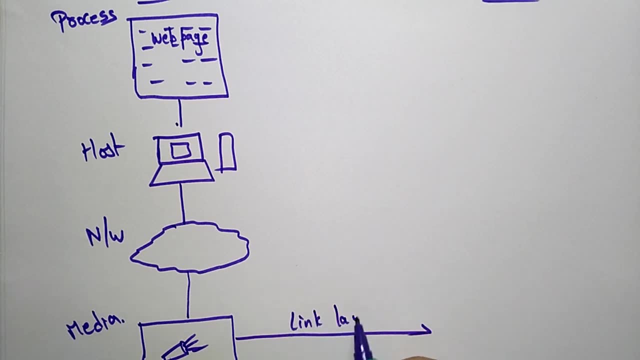 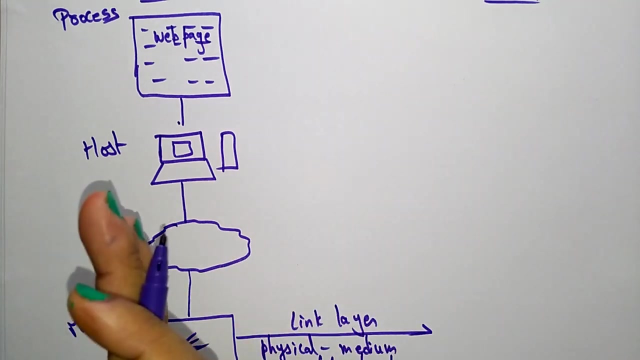 Okay, So here, with the help of the media, that is, the link layer. So this is a physical medium independent. So the servers, the client side and the server side, whatever the physical medium that we are using that may be independent to each other. 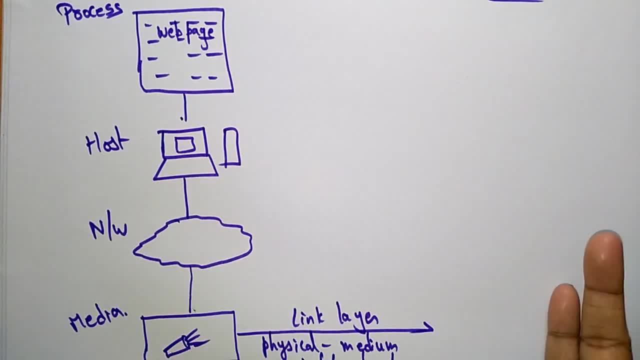 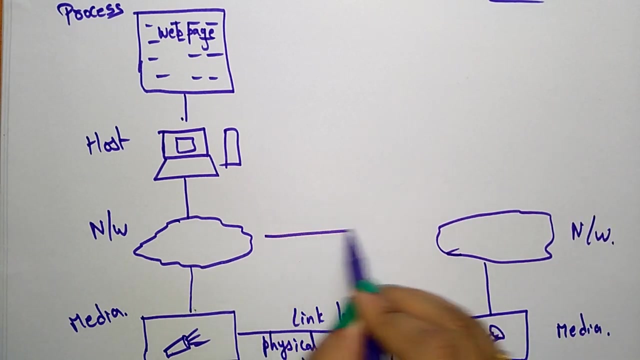 So here we use, suppose, some another cable and here we are using some wireless or whatever it may be. The medium is different from one system to the another system, So it is independent. This is a medium And here this is a network. So communication between these two networks is in, you call it as in a network. 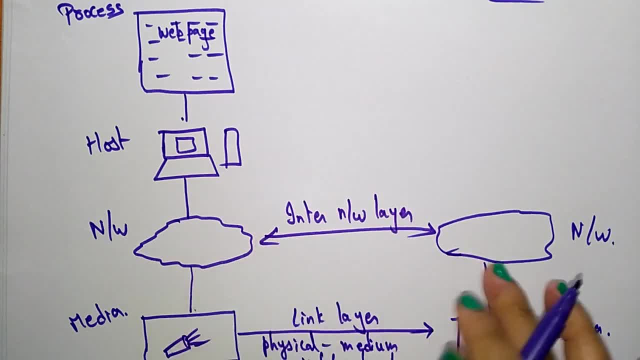 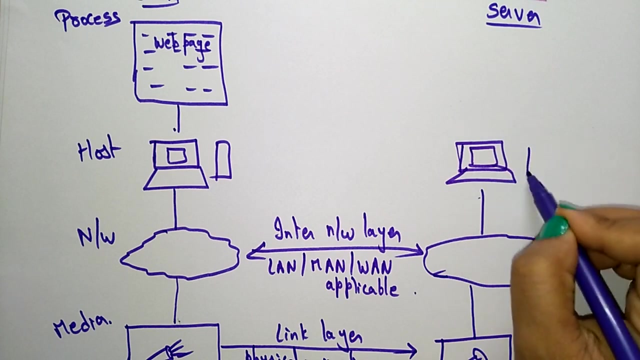 And here this is an inter network, This is an inter network layer, So the inter network layer. we use the LAN or MAN or WAN, So these three networks are applicable. So next it reaches the host. So this is a host, So a communication between the client and server.